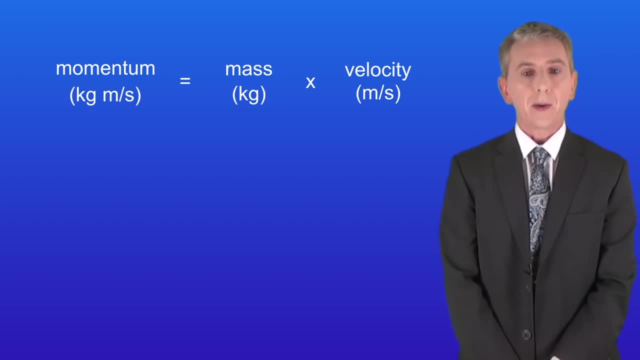 We calculate momentum using this equation: Momentum equals the mass multiplied by the velocity. Remember that in a closed system, the total momentum before an event is equal to the total momentum after an event. In other words, momentum is always conserved. So in this video, we're going to use the conservation of momentum to carry out calculations involving 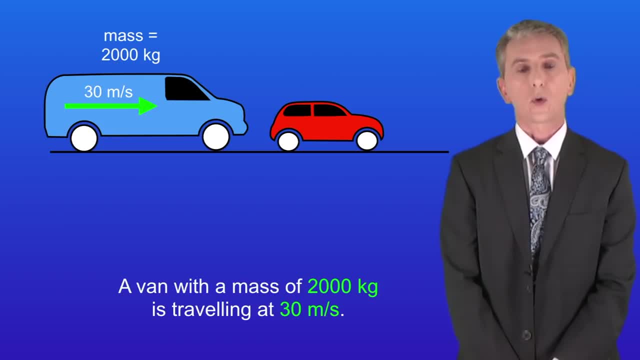 an event such as a collision. Here's a sample question. A van with a mass of two thousand kilograms is travelling at thirty metres per second. It collides with a stationary car with a mass of eight hundred kilograms. Both the van and the car continue moving together. Calculate the velocity of the van and the. 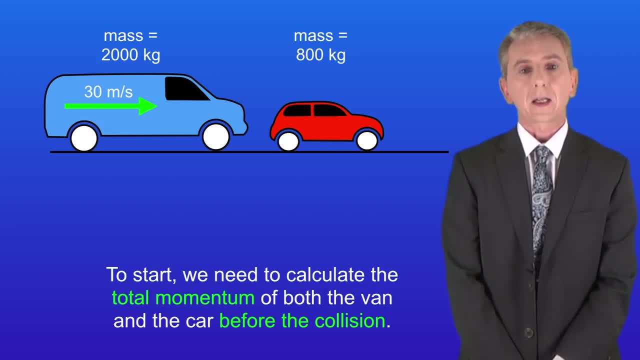 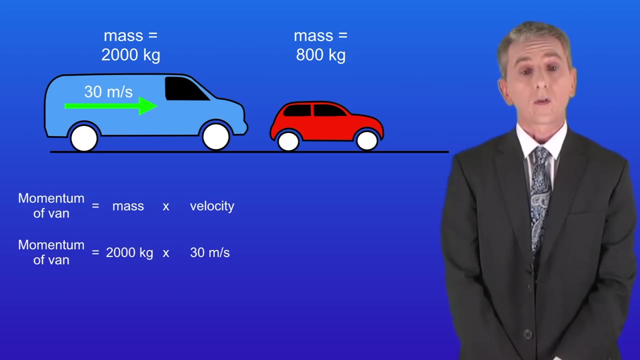 car together. So to start, we need to calculate the total momentum of both the van and the car before the collision. We're going to start with the van. Remember that momentum equals the mass multiplied by the velocity. The mass of the van is two thousand kilograms and the velocity is thirty. 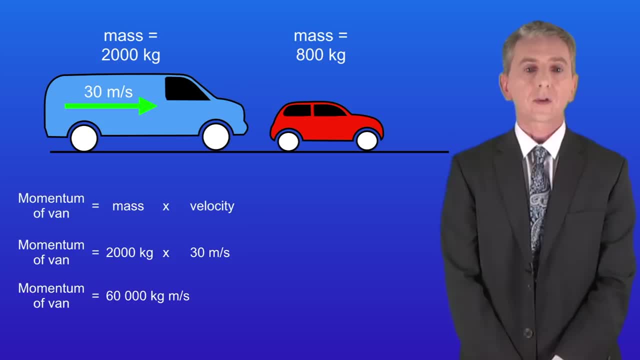 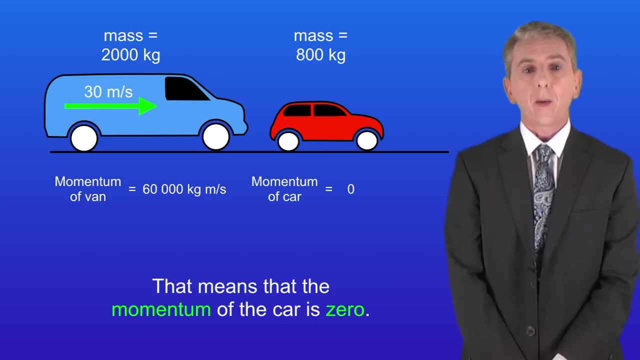 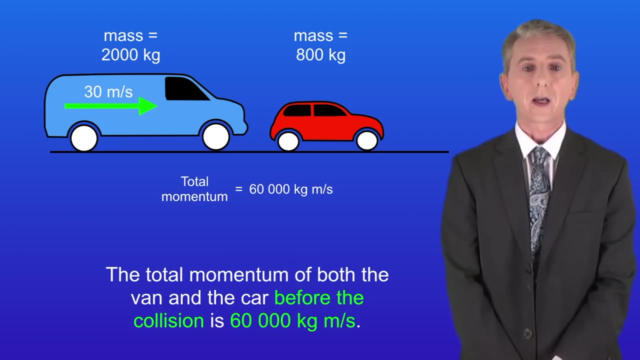 metres per second. That gives us a momentum of sixty thousand kilograms metre per second for the van. Looking at the car, we can see that the car is stationary. That means that the momentum of the car is zero. So the total momentum of both the van and the car before the collision is sixty thousand. 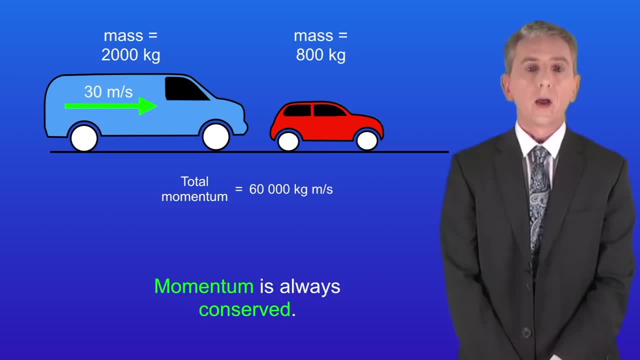 kilograms metre per second. As we saw before, momentum is always conserved, So that means that the total momentum of the van and the car after the collision is also sixty thousand kilograms metre per second. We can use this to calculate the velocity of the van and the car together. Remember. 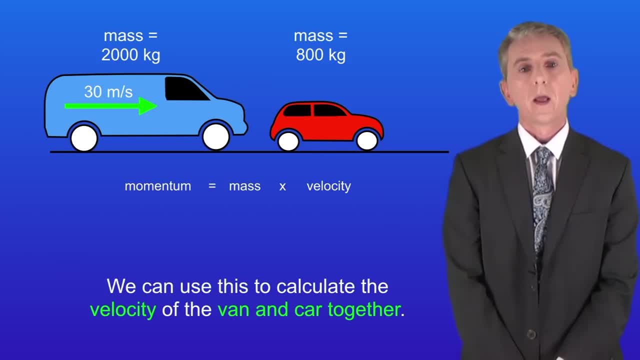 that momentum equals the mass multiplied by the velocity. That means that the velocity equals the momentum divided by the mass. The momentum after the collision is sixty thousand kilograms metre per second, and the total mass of both the van and the car is two thousand eight hundred kilograms. 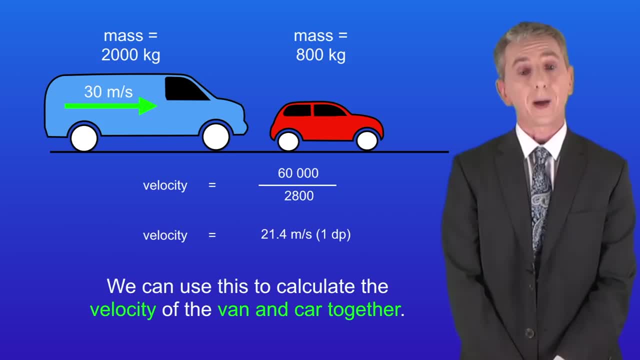 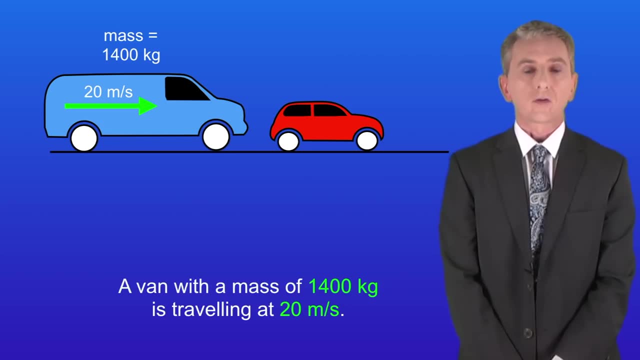 Putting these into the equation gives us a velocity of the car and the van combined of twenty one point four metres per second. So that means that the total weight of both the meters per second to one decimal place- Here's a question for you- to try A van. 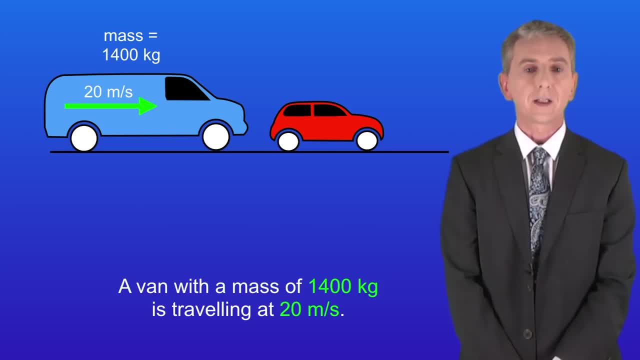 with a mass of 1,400 kilograms, is traveling at 20 meters per second. The van collides with a stationary car with a mass of 1,000 kilograms. Both the van and the car continue moving together. Calculate the velocity of the van and.